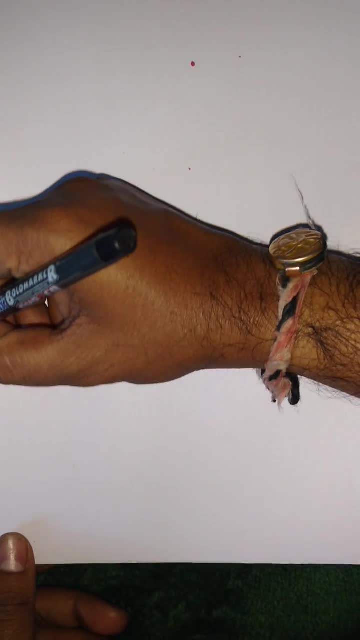 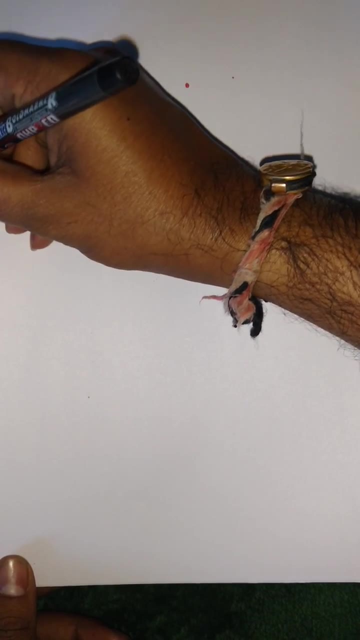 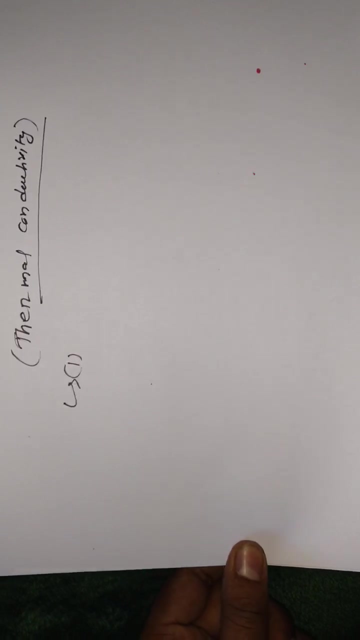 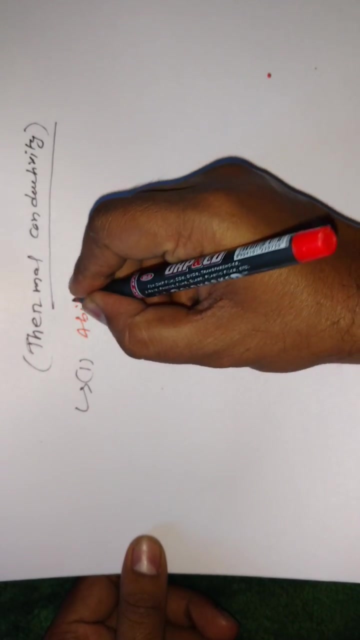 Hi, my dear, this is a very short video. In this video, I will share with you about thermal conductivity. Thermal conductivity, Right, As you know, thermal conductivity. here I am going to do like this point wise. That's why you can understand about it. Okay, Now, what is thermal conductivity? basically, Thermal conductivity is something which is having ability, Ability of the material, of the material. 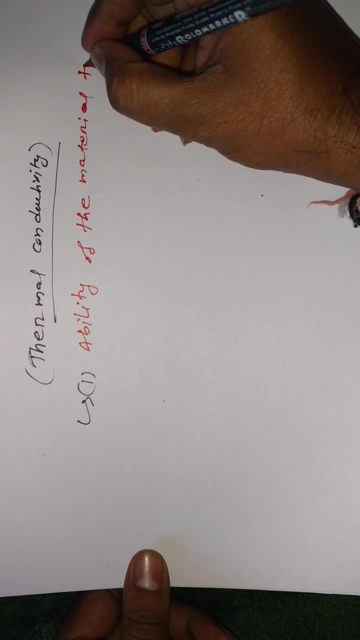 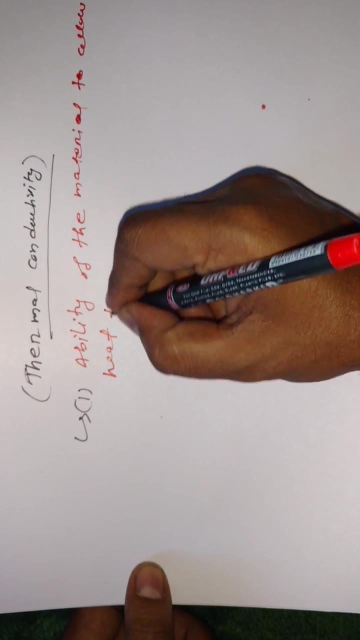 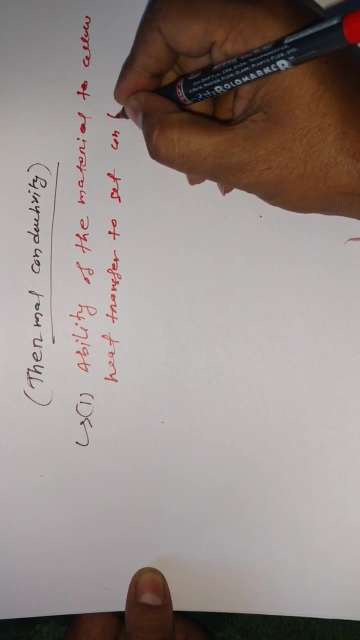 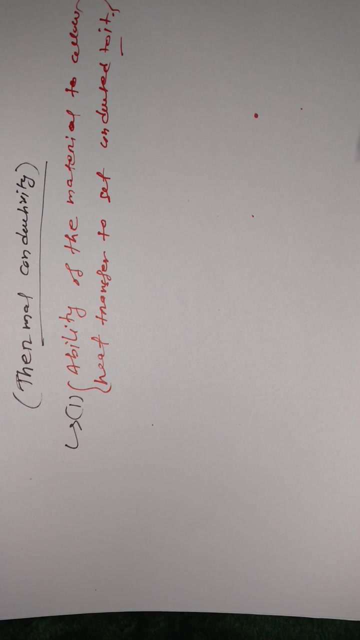 Material to material to allow, to allow heat transfer. heat energy or heat transfer must say heat energy transfer to get conducted to it, Right. So thermal conductivity is something which is which allow to heat transfer of a solid or liquid mummy gas. because there are three: process where conduction, process with their 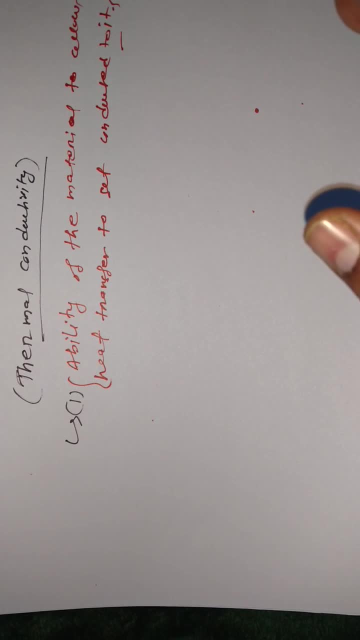 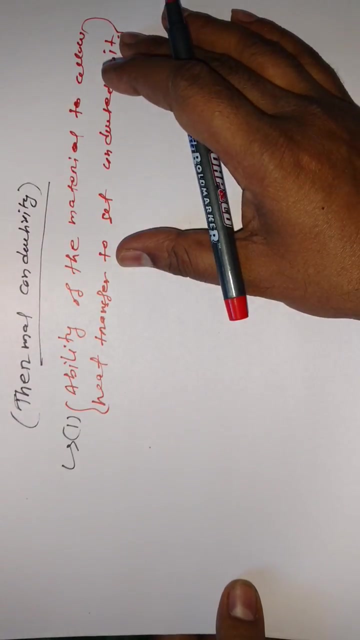 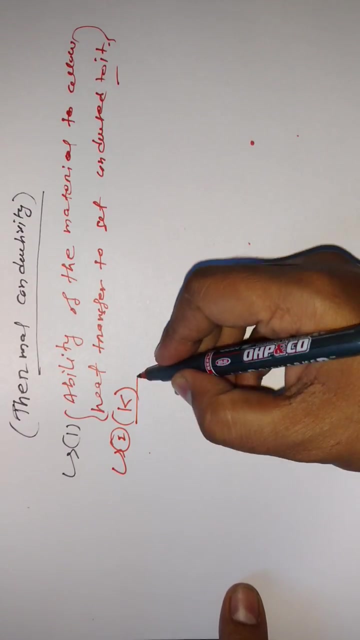 in all of the matter, three types of matter: solid, liquid and gas. in all of the matter, conduction process can takes place. I have already shared and I will also explain all those things in my next video. But today, thermal conductivity, what is? I have already shared with you. now, What is the unit of thermal? I mean how we can denote thermal conductivity, that is, we can denote thermal conductivity by key. Now, third, what is the unit of thermal conductivity? 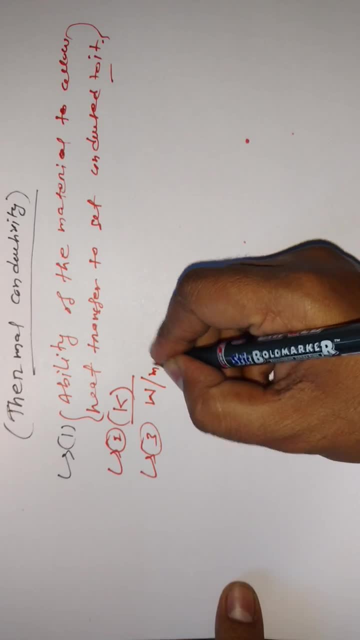 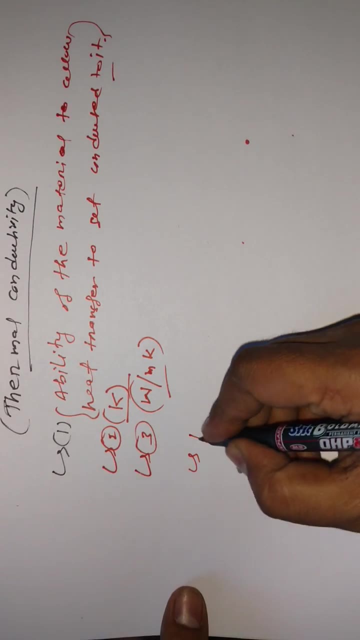 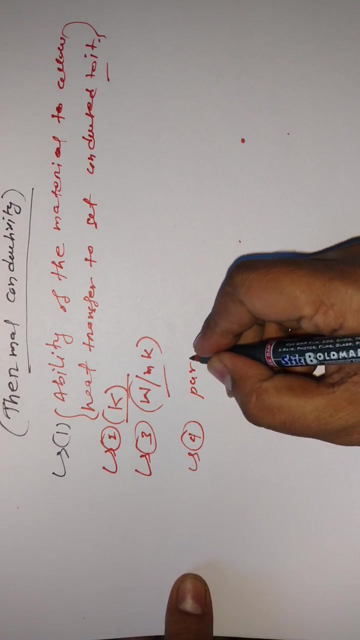 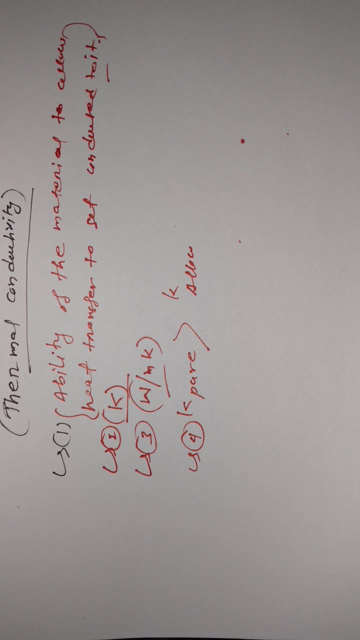 Thermal conductivity, that is what per meter Kelvin? All these three things are most important in case of thermal conductivity. And one more thing, one more thing: Right, If there are two, two particles or two substance- I must say one is PO and another one is alloy- Then thermal conductivity of PO is always greater than thermal conductivity of alloy. If you wanted to know example, then thermal conductivity of alloy is always greater than thermal conductivity of alloy. 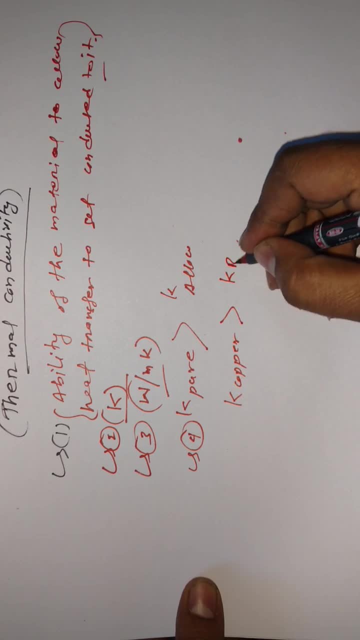 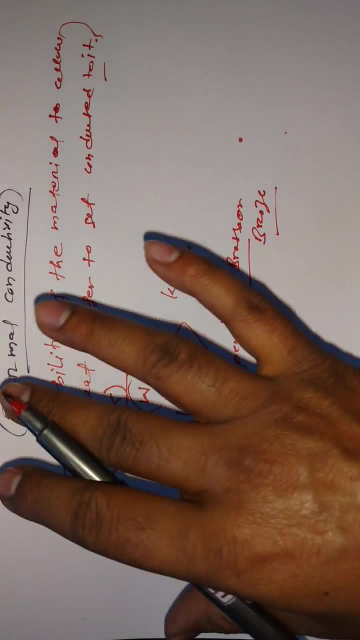 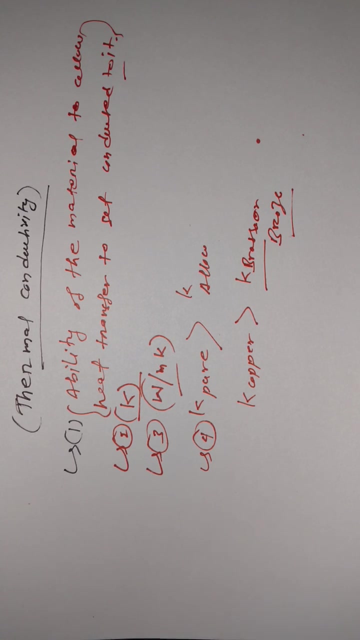 If you wanted to know example, then thermal conductivity of copper is always greater than thermal conductivity of brass or bronze or bronze, because brass is also known as bronze. So this is all about thermal conductivity. I hope you understand some basic concept about the thermal conductivity. So in my next lecture I will share with you a couple of more videos related to conduction. Hope you are enjoying heat and mass transfer. Thanks.